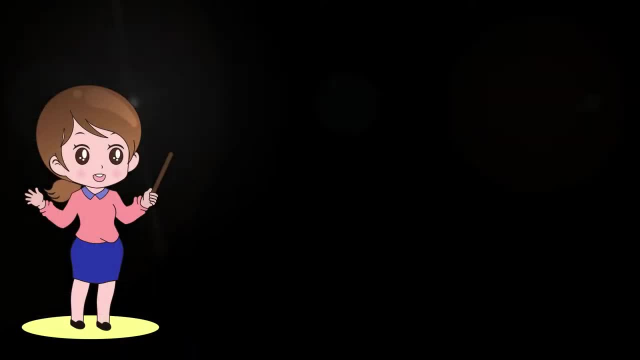 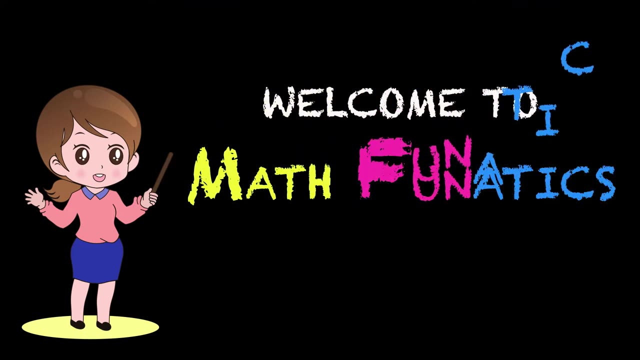 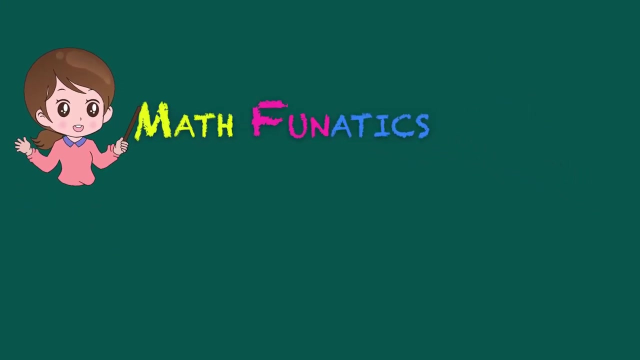 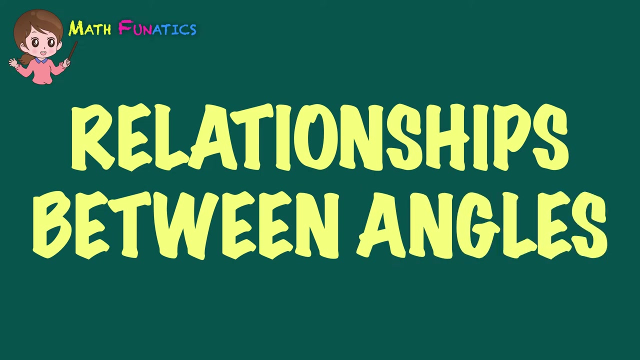 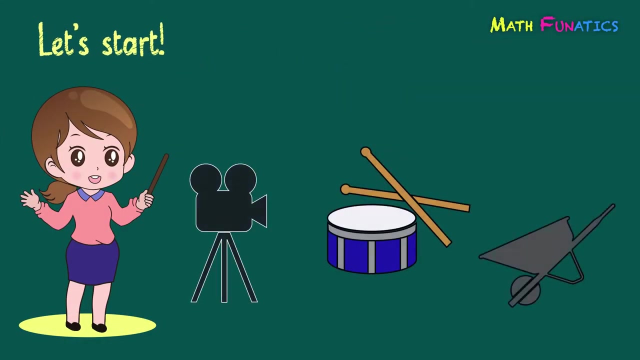 Welcome to Math Fanatics. In this video we're going to learn about Relationships Between Angles. After learning the parts and different kinds of angle from our previous video, let us learn more about the different relationships between angles. Let's start by taking a look at the following illustrations: 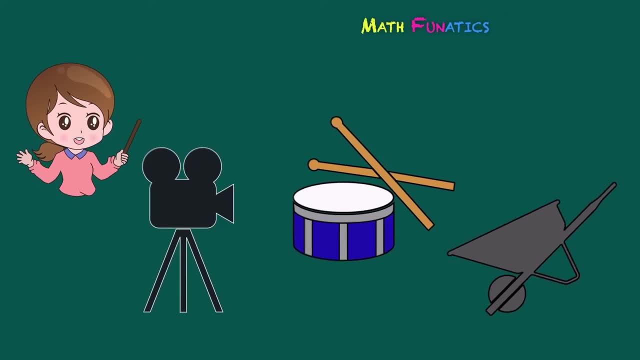 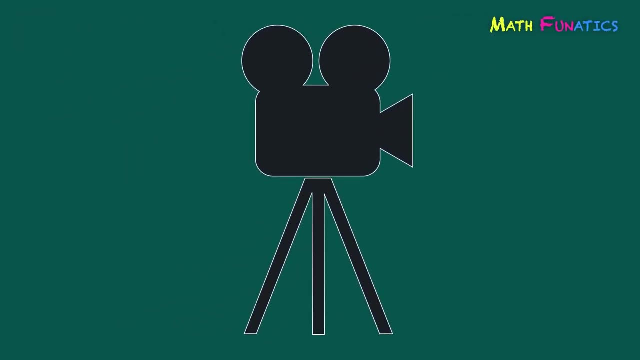 Observe carefully and look for the angles that are shown in each illustration. The first illustration is a camera mounted on a tripod stand. Do you see angles in this illustration? That's right, There are two angles placed side by side, as seen in the tripod stand. 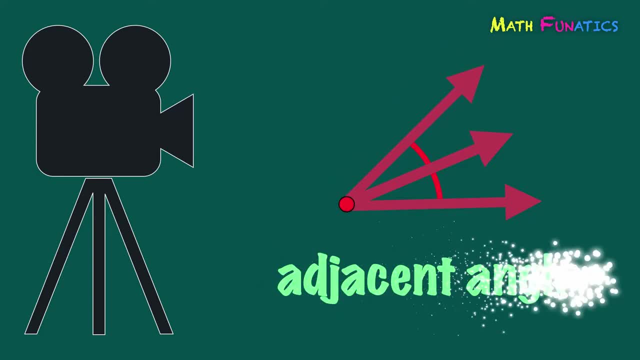 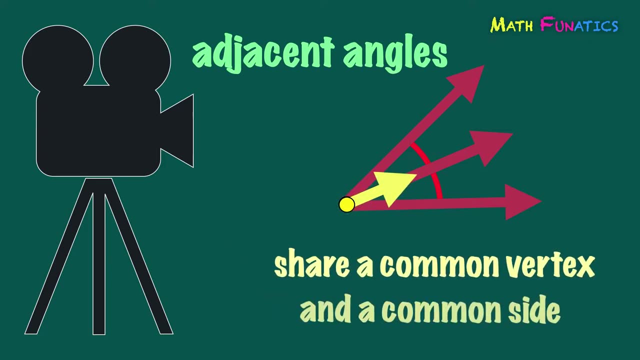 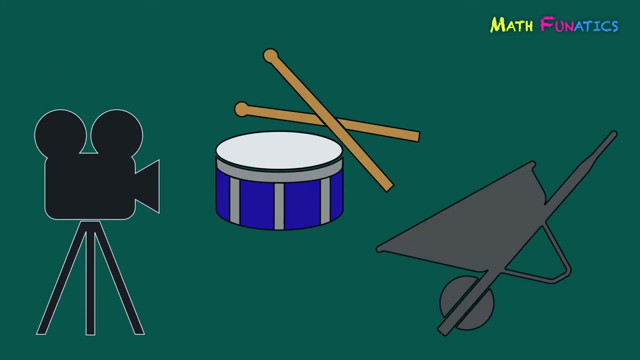 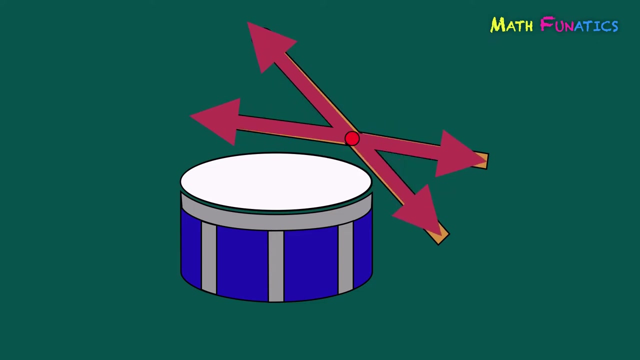 These two angles are called adjacent angles. Observe that adjacent angles share a common vertex and a common side. Again, these are adjacent angles. Next illustration shows a drum with a pair of drumsticks. Now the angles are found on the opposite directions of the overlapping pair of drumsticks. 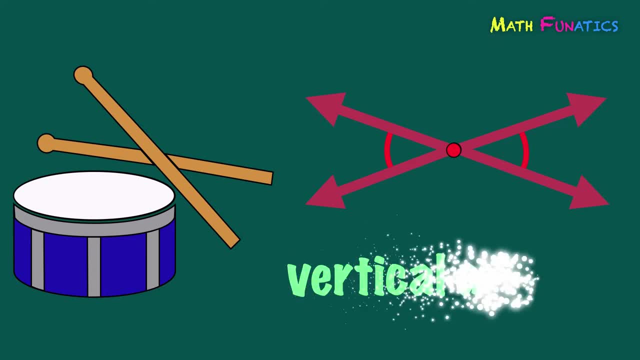 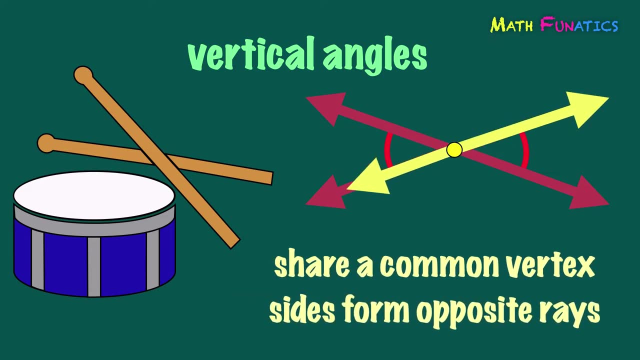 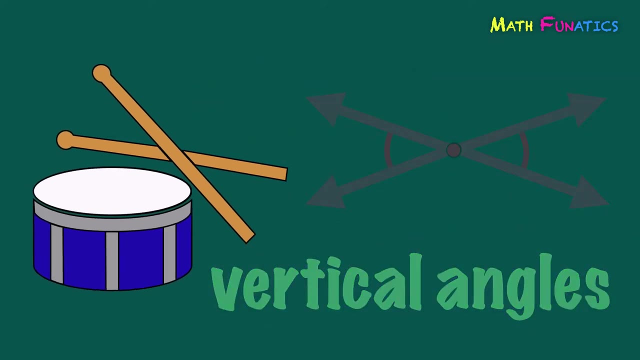 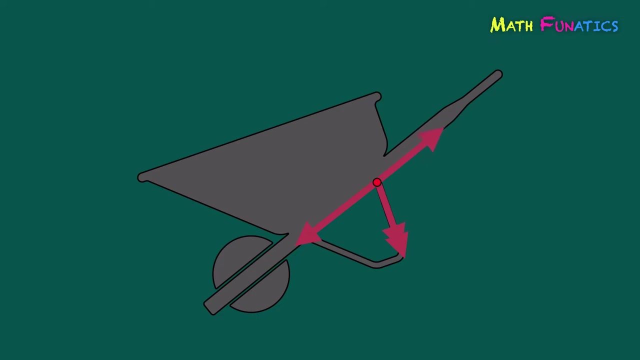 These two angles are called vertical angles. Observe that vertical angles share a common vertex and their sides form opposite rays. Again, these are vertical angles. The last illustration shows a wheelbarrow. We see that the angles are also placed side by side. 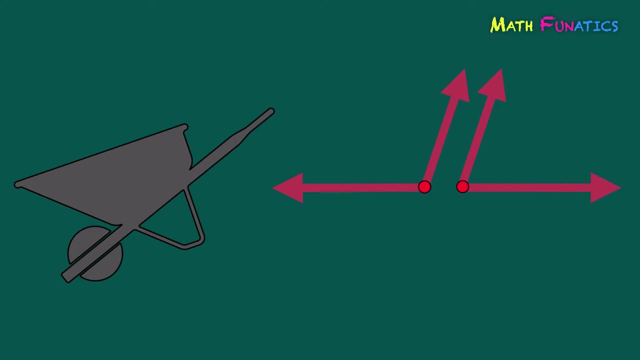 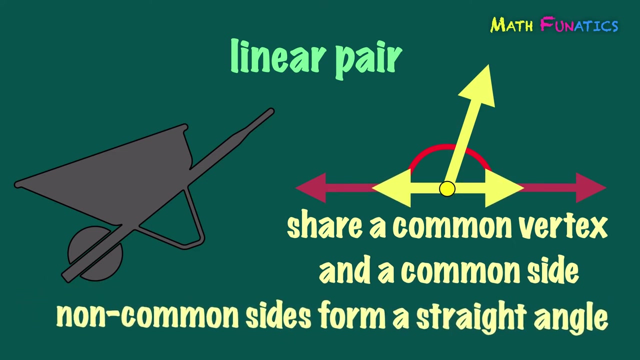 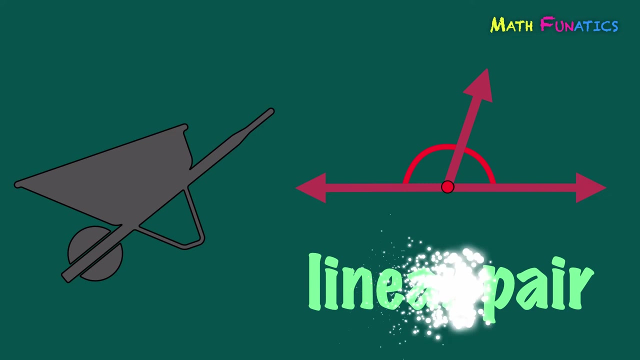 These two angles are adjacent angles that form a linear pair. Notice that the angles forming a linear pair share a common vertex and a common side. In addition to that, their non-common sides form a straight angle. Again, these angles form a linear pair. 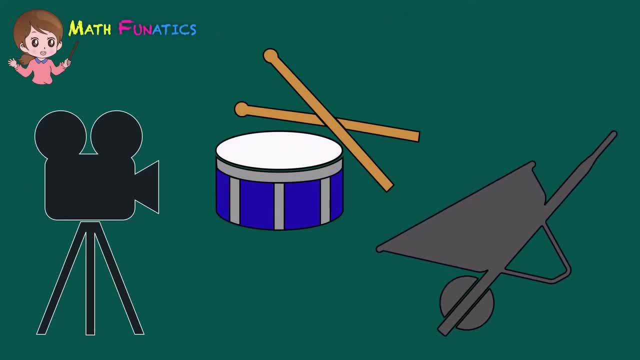 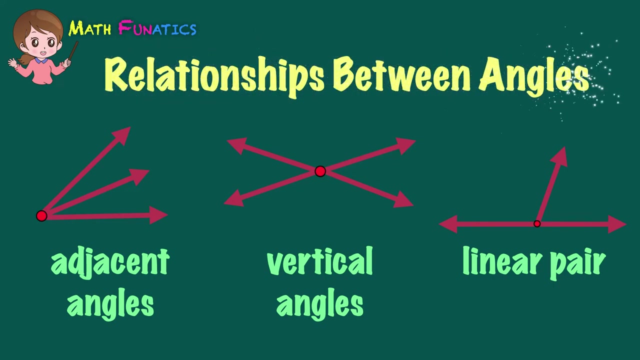 Let's go back to the three illustrations. The tripod of the camera shows adjacent angles, while the drumsticks show vertical angles and the wheelbarrow illustrates angles forming a linear pair. All these three pairs of angles show the relationships between angles. Now let's practice what you've learned today. 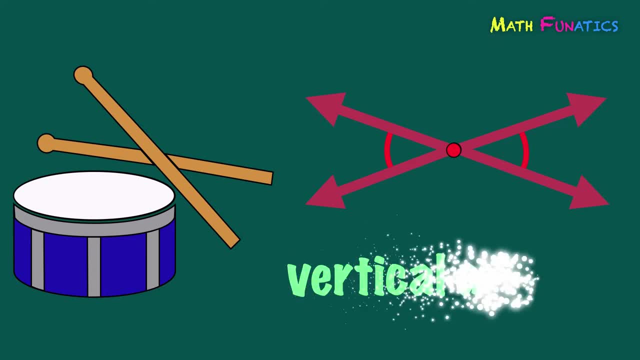 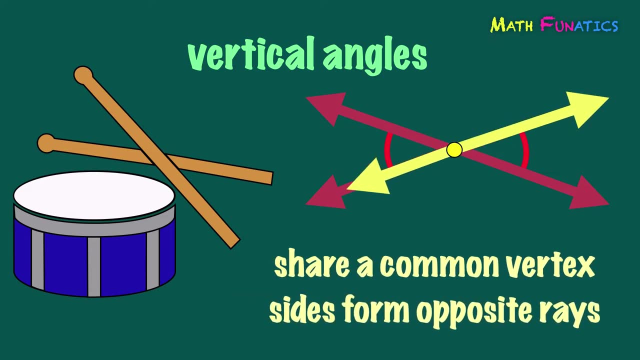 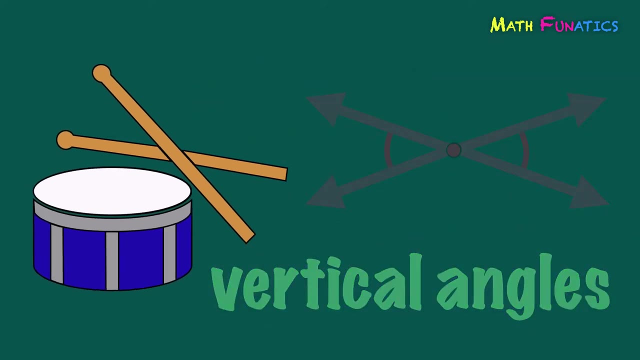 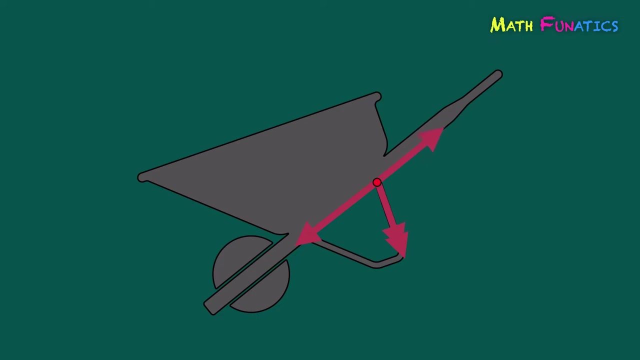 These two angles are called vertical angles. Observe that vertical angles share a common vertex and their sides form opposite rays. Again, these are vertical angles. The last illustration shows a wheelbarrow. We see that the angles are also placed side by side. 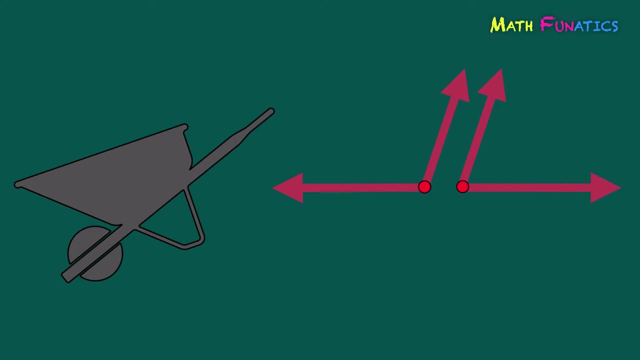 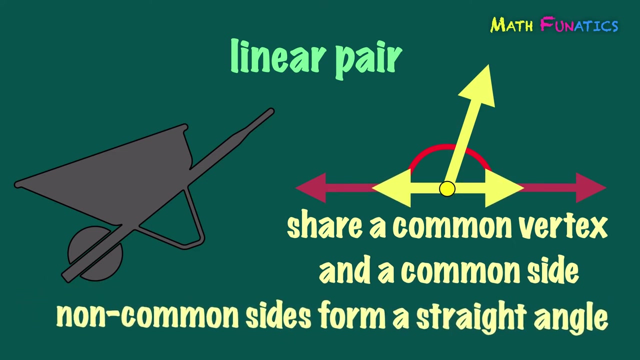 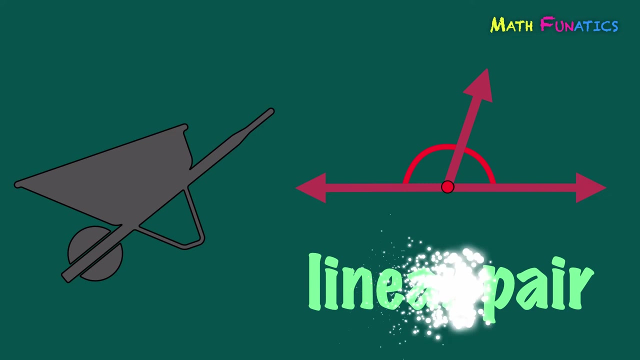 These two angles are adjacent angles that form a linear pair. Notice that the angles forming a linear pair share a common vertex and a common side. In addition to that, their non-common sides form a straight angle. Again, these angles form a linear pair. 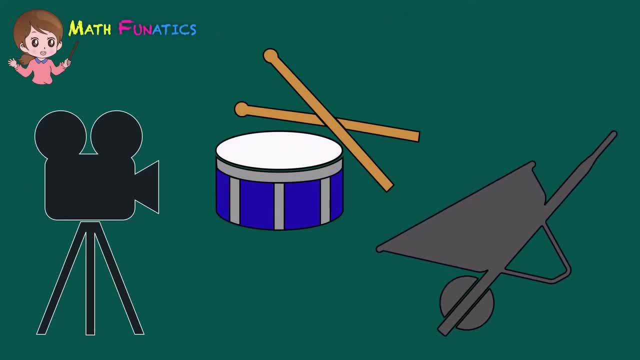 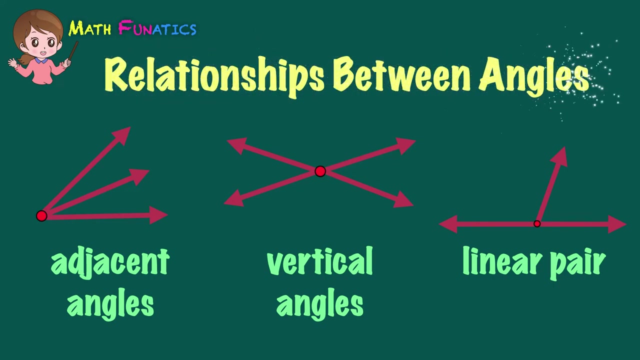 Let's go back to the three illustrations. The tripod of the camera shows adjacent angles, while the drumsticks show vertical angles and the wheelbarrow illustrates angles forming a linear pair. All these three pairs of angles show the relationships between angles. Now let's practice what you've learned today. 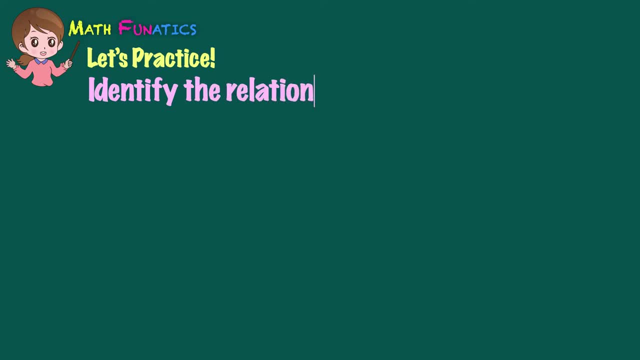 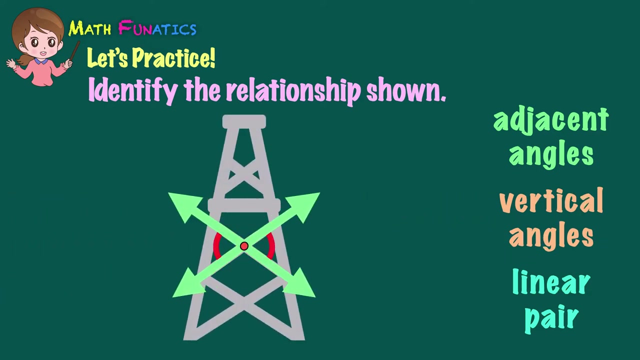 Identify the relationships shown. Tell if the angles are adjacent, vertical or form a linear pair. Here's the first question: What is the relationship shown by the angles of the tower? I am giving you five seconds to think. What's your answer? 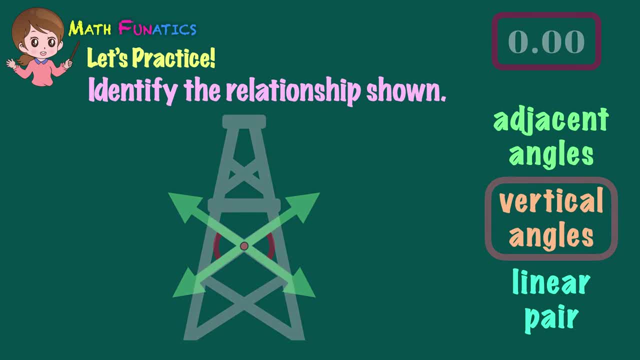 That's right, They're vertical angles. Next, what is the relationship shown by the angles of the compass? What's your answer? Correct, They form a linear pair. This time, what is the relationship shown by the angles of the satellite dish?